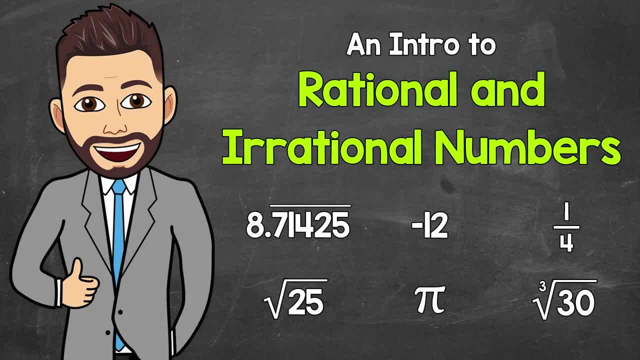 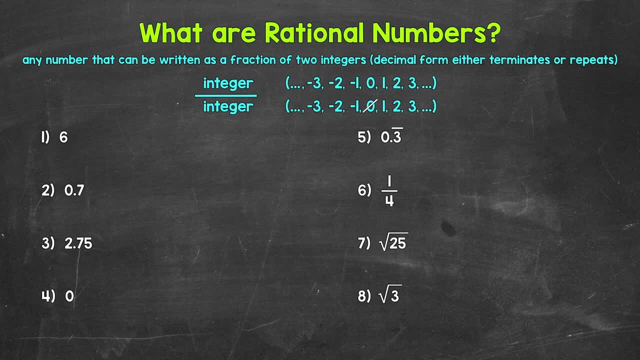 Welcome to Math with Mr J. In this video I'm going to go through an introduction to rational numbers and irrational numbers. We'll start with rational numbers and then move on to irrational numbers. Now, simply put, rational numbers are numbers that can be written as a fraction. 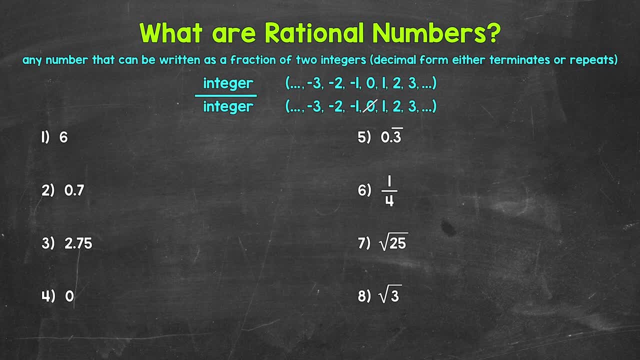 specifically a fraction of two integers. So the numerator must be an integer and the denominator must be an integer. Now fractions can be written as decimals, so anything in decimal form that either terminates, so cuts off, or repeats, so continues on forever in some type of pattern. 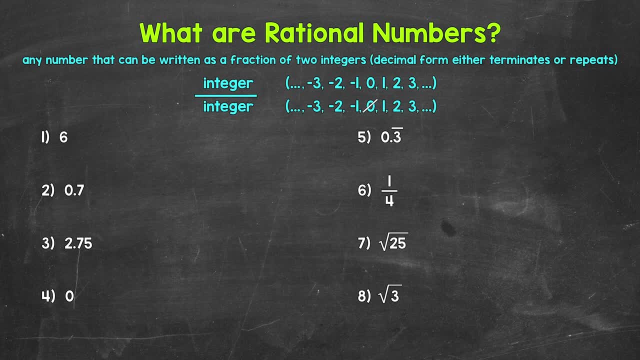 those are rational numbers. This may all seem confusing at first, but as we go through our examples this will all make a lot more sense. So any number that can be written as a fraction of two integers. so the numerator must be an integer and the denominator must be an integer. 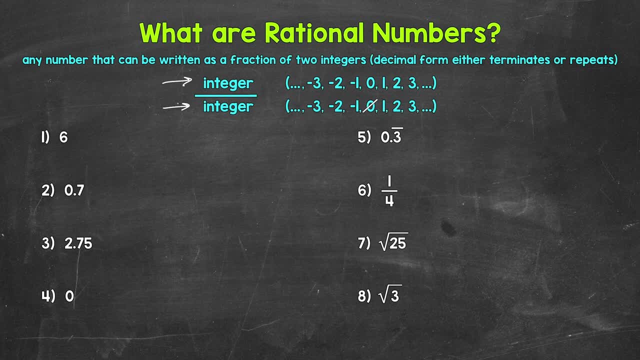 that's going to be a rational number. Now remember: integers include positive and negative numbers and zero. Decimals and fractions are not included. Now, one thing I do want to mention: the denominator cannot be zero, because that will give us a value that is undefined. That's why zero is crossed off for the denominator. So something to keep in mind. 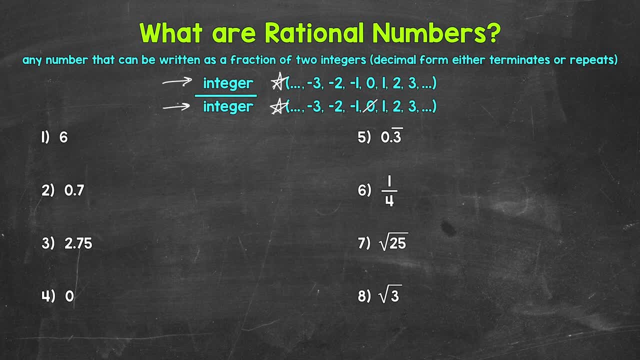 Let's jump into our examples, starting with number one, where we have six. So we have a whole number here. Can we write six as a fraction of two integers? Yes, For example, we can write six over one- That equals six, Or 12 over two- That equals six. 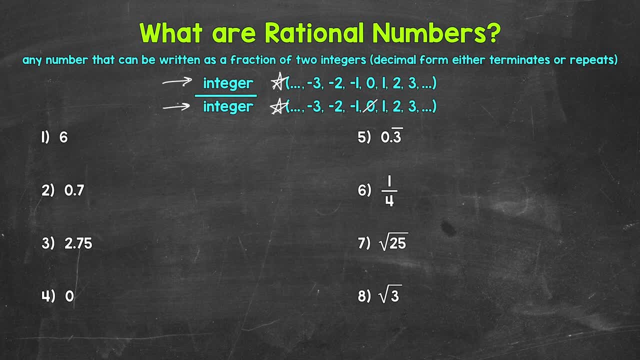 Let's jump into our examples, starting with number one, where we have six. So we have a whole number here. Can we write six as a fraction of two integers? Yes, For example, we can write six over one- That equals six, Or 12 over two- That equals six. 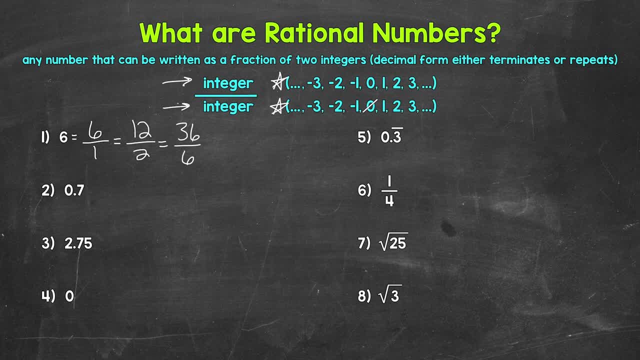 Or we can write six over six. That equals six. All of those examples equal six. So six can be written as a fraction of two integers. so it's a rational number And ALL whole numbers are going to be rational. What about negative six? What about a negative number? 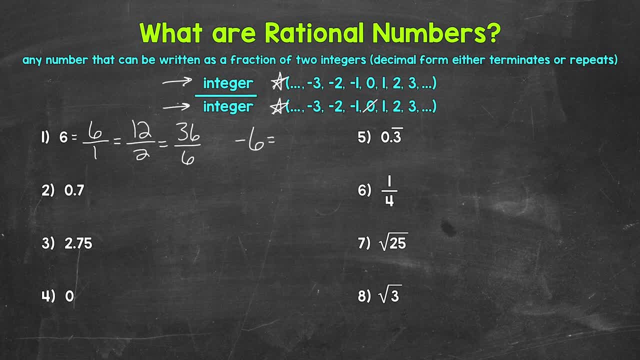 Can we write this as a fraction of two integers? Yes, Negative six over one equals negative six. Or negative eighteen over three equals negative six, 6.. So negative 6 is a rational number as well. Let's move on to number two, where we have a. 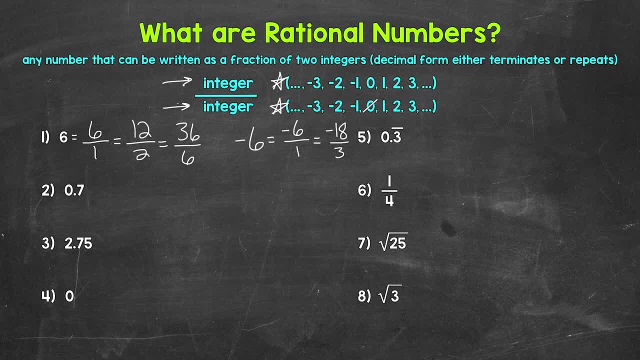 decimal 7 tenths. Is this rational? Well, it is a terminating decimal, It cuts off. So right away we can see that this is rational. But can it be written as a fraction of two integers? Yes, 7 tenths can be written as 7 over 10.. That equals 7 tenths. Or 21 over 30 equals 7 tenths. 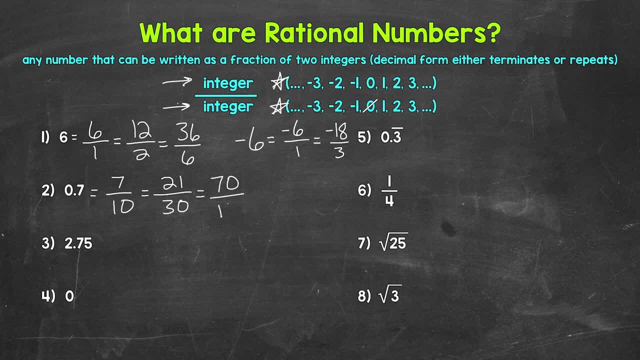 Or even 70 over 100 equals 7 tenths. So 7 tenths can be written as a fraction of two integers. So it's rational. And just like we talked about number one- a negative, so negative 7 tenths can be written as a fraction of two integers. So it's rational, And just like we 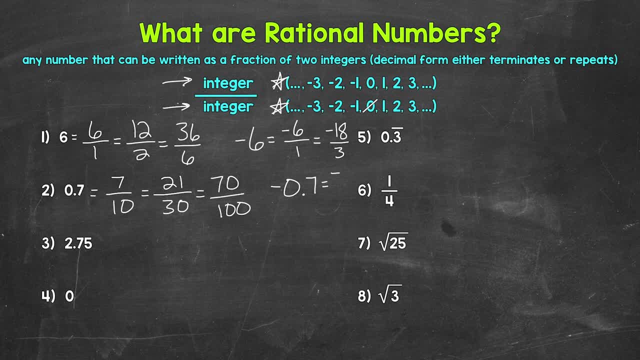 that's rational as well. We can write this as negative 7 tenths, So any terminating decimals are going to be rational. Let's move on to number three, where we have 2 and 75 hundredths. Similar to number two. we have a terminating decimal, So right away we can tell that this. 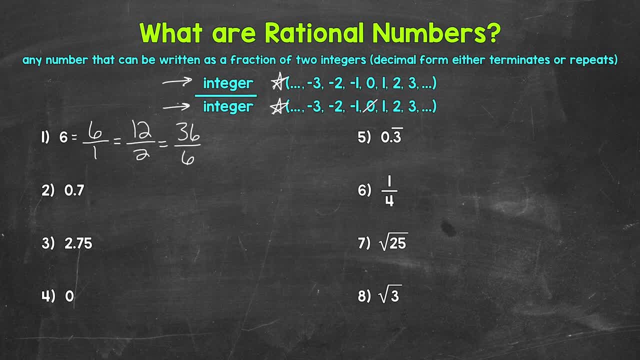 Or 12 over two, That equals six. Or 12 over two, That equals six. All of those examples equal six. So six can be written as a fraction of two integers. So it's a rational number And all whole numbers are going to be rational. 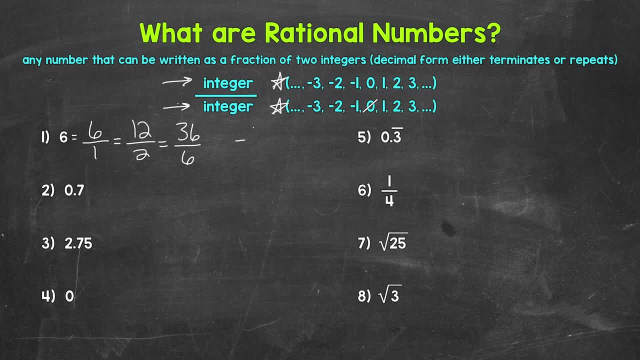 What about negative six? What about a negative number? Can we write this as a fraction of two integers? Yes, Negative six over one equals negative six. Or negative eighteen over three equals negative six. Or negative eighteen over three equals negative six. So negative six is a rational number as well. Let's move on to number two, where we have a. 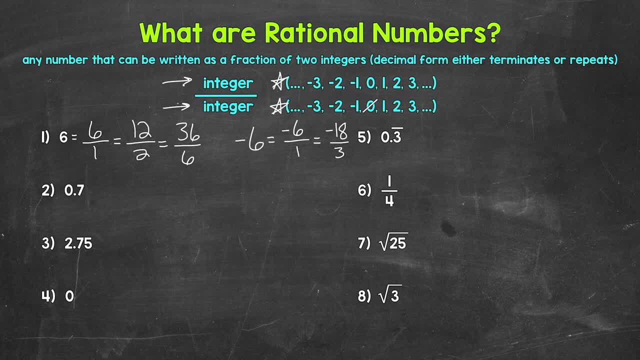 decimal Seven tenths. Is this rational? Well, it is a terminating decimal, It cuts off. So right away we can see that this is rational. But can it be written as a fraction of two integers? Yes, Seven tenths can be written as seven over ten. That equals seven tenths, Or. 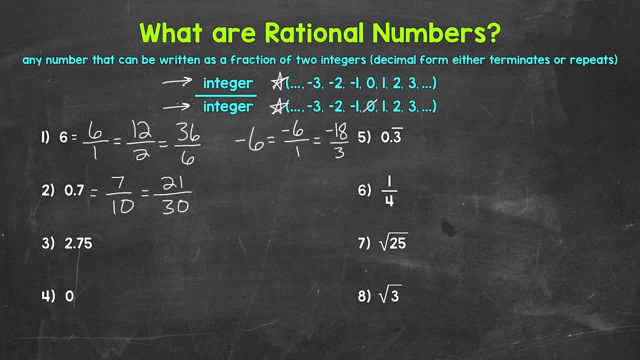 even thee. So absolutely So. seven tenths can be written as a fraction of two integers, So it's rational as well. Boom, Just like we spoke about number one, There is a declaration, So a negative seven tenth. I'm sending both, sounds, guess. 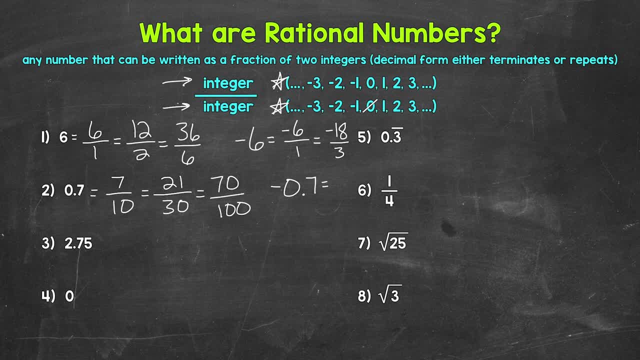 So negative seven tens. That is rational as well. Can we have a statement as a negative seven tens? and thecro James and tell us what we know about it? There is a statement as a fraction of two integers, Which is from Or procedures, So from, and also an. 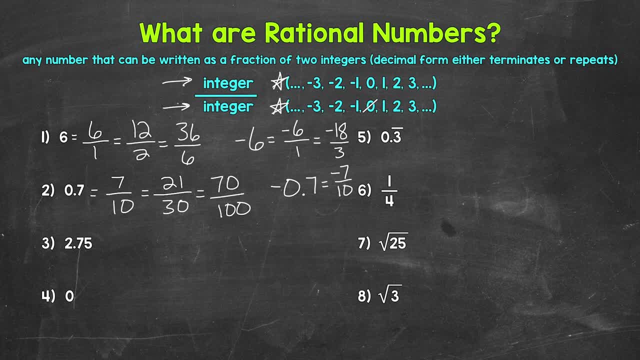 operating language of Mister Jackson and possible option of stadem q, which is what we have think about. the decimals are going to be rational. Let's move on to number three, where we have two and 75 hundredths Similar to number two. we have a terminating decimal, so right away we can tell that this: 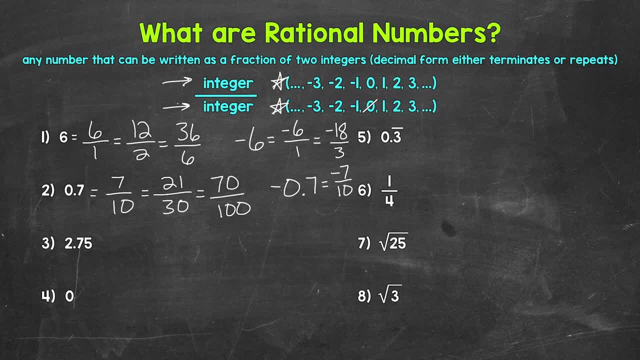 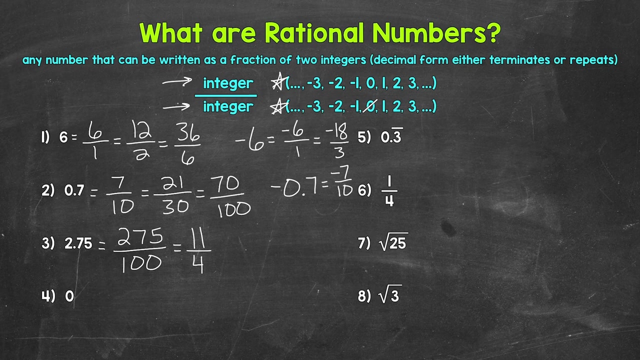 is rational. But how do we write this as a fraction of two integers? Well, we can write this as 275 over 100.. Or we can even use the simplified version of that fraction: 11 over 4.. So both of those are examples of two and seventy five hundredths written as a fraction of two. 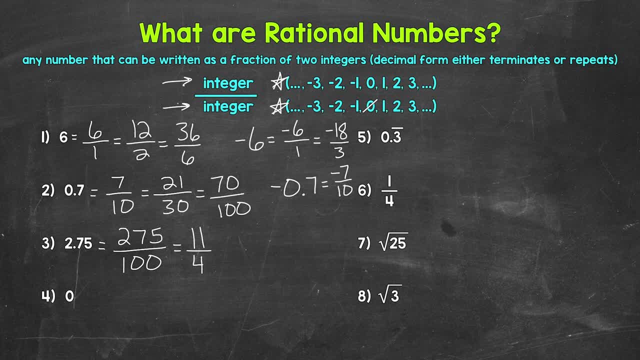 integers. Now, just like numbers one and two, negative two and seventy five hundredths is rational as well. We can write that as a fraction of two integers. a fraction of two integers. Let's move on to number four. where we have zero, Is zero rational? 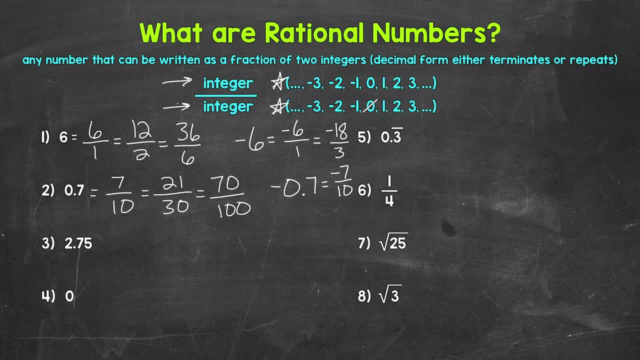 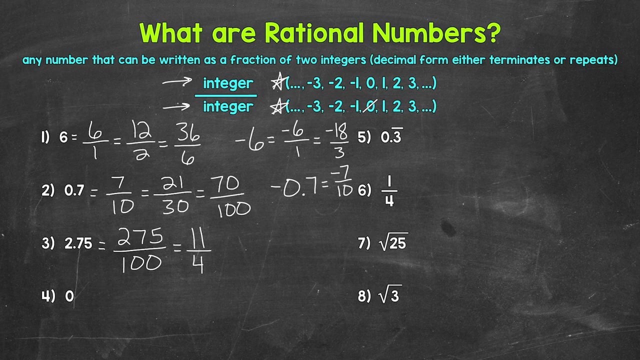 is rational. But how do we write this as a fraction of two integers? Well, we can write this as 275 over 100.. Or we can even use the simplified version of that fraction: 11 over 4.. So both of those are examples of 2 and 75 hundredths written as a fraction of two integers. Now, 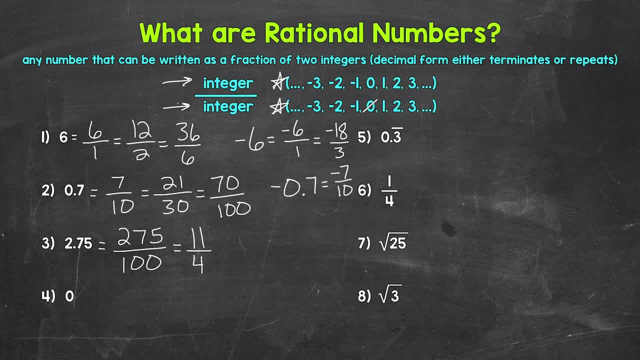 just like numbers 1 and 2, negative 2 and 75 hundredths is rational as well. We can write that as a fraction of two integers. Let's move on to number four, where we have 0.. Is 0 rational? 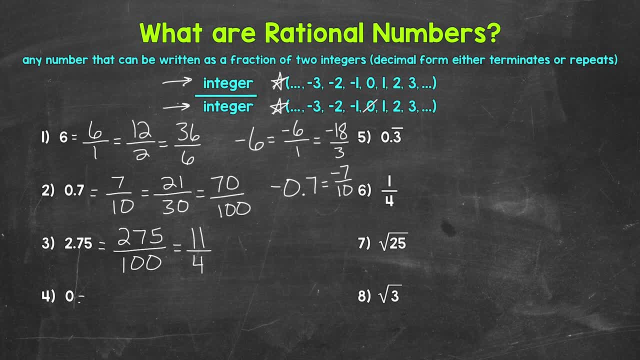 Yes, we can write 0 as a fraction of two integers. 0 over 1 equals 0.. 0 over 25 equals 0.. 0 over 100 equals 0.. So, yes, we can write 0 as a fraction of two integers. 0 is. 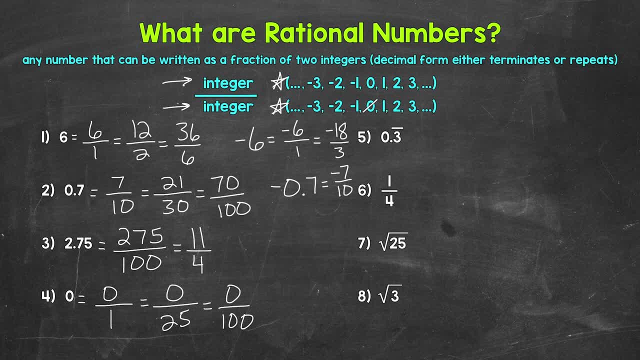 is rational. Now, like I mentioned earlier in the video, if we have 0 in the denominator, though- so let's just say 1 over 0,- this does not equal 0.. 0 in the denominator gives us a value, that is. 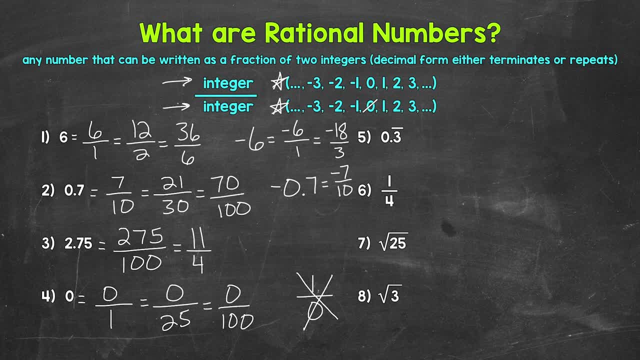 undefined. So that's not going to be rational. So again something to keep in mind. Let's move on to number five, where we have a repeating decimal, So 0.3. repeating This bar right here, this means we have 0.3 and this 3 continues on forever. So is this rational? Are repeating? 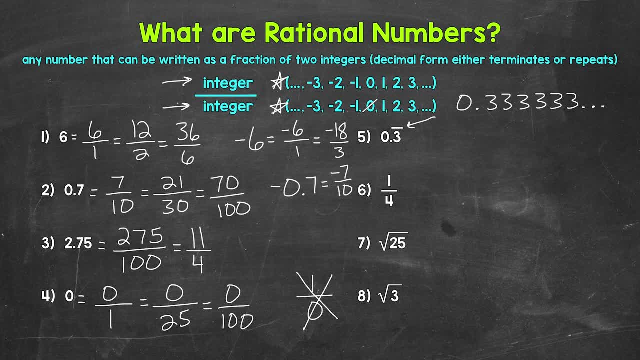 decimals rational. Can we write this as a fraction of two integers? Yes, we can actually write any repeating decimal as a fraction of two integers. For example, a fraction of two integers that equals 0.3 repeating Well, one third. 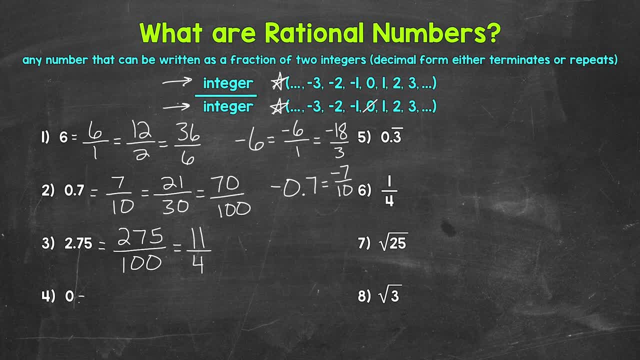 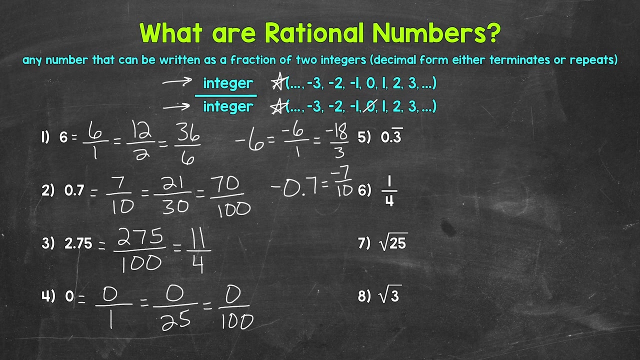 Yes, we can write zero as a fraction of two integers. Zero over one equals zero. Zero over 25 equals zero. Zero over 100 equals zero. So, yes, we can write zero as a fraction of two integers. Zero is rational. Now, like I mentioned earlier in the video, if we have zero, 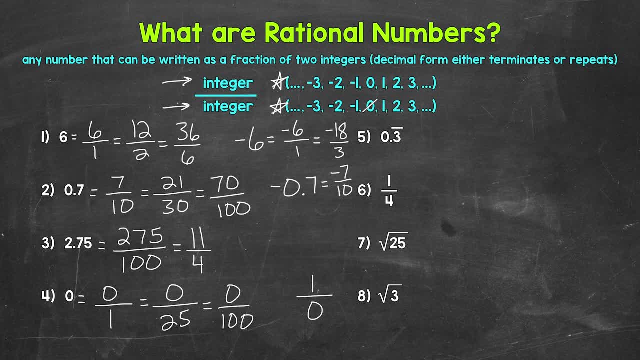 in the denominator though. so let's just say one over zero. this does not equal zero. Zero in the denominator gives us a value that is undefined, So that's not going to be rational. So again, something to keep in mind. Let's move on to number five, where we have a repeating decimal, So 0.3. 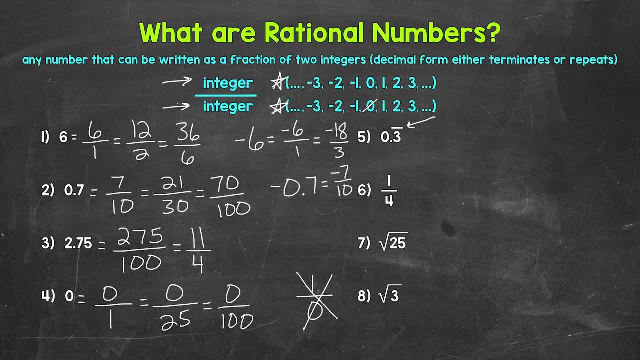 repeating This bar right here, this means we have 0.3 and this 3 continues on forever. So is this rational? Are repeating decimals rational? Can we write this as a fraction of two integers? Yes, we can actually write any repeating decimal as a fraction of two integers. 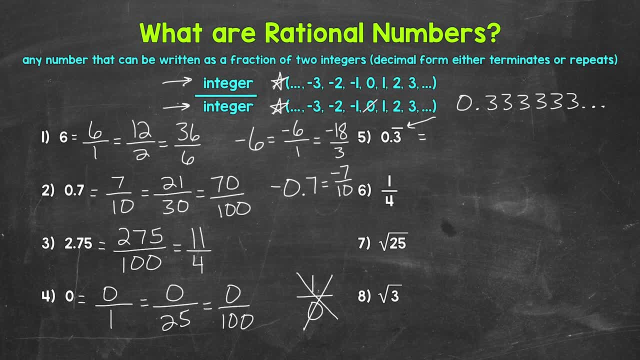 For example, a fraction of two integers, that equals 0.3 repeating. Well, one third or three ninths. So any repeating decimals are rational, Even something that has multiple digits that repeat will be rational. So, for example, something like 0.181818 and this: 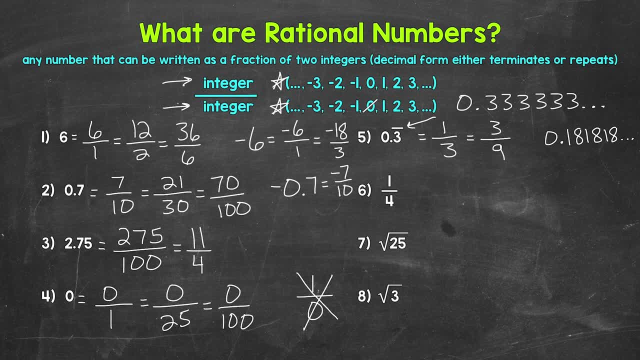 continues on. So 18 repeating. We have a pattern here, We have something that repeats. So this is rational Fractional form. let's come below here. So 0.18 repeating. We can do 18 over 99 or even 2 over 11.. 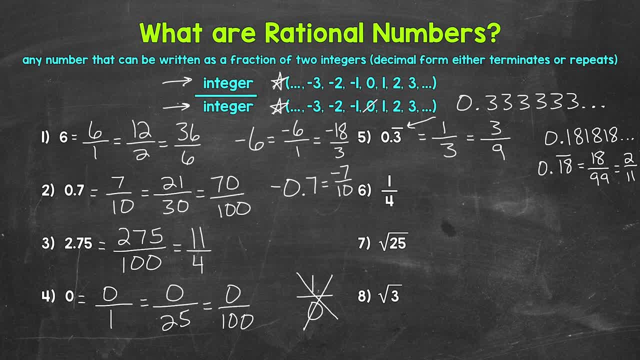 Next, for number six, we have one fourth. Well, this is already a fraction. The numerator is one, which is an integer, and the denominator is four, which is an integer. So this is rational. Now let's look at the decimal form as well. One fourth equals 25 hundredths, which is a 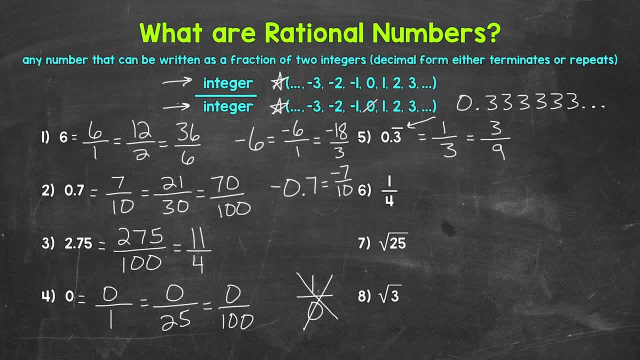 Or three ninths. So any repeating decimals are rational. Even something that has multiple digits that repeat will be rational. So, for example, something like 0.181818 and this continues on, So 18 repeating. We have a pattern here, We have something that repeats. So this is rational. 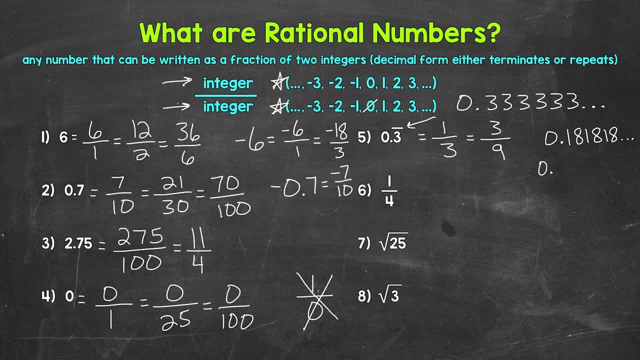 Fractional form. Let's come below here. So 0.18. repeating, We can do 18 over 99.. Or even 2 over 11.. Next, for number six, we have one fourth. Well, this is already a fraction. The numerator is one. 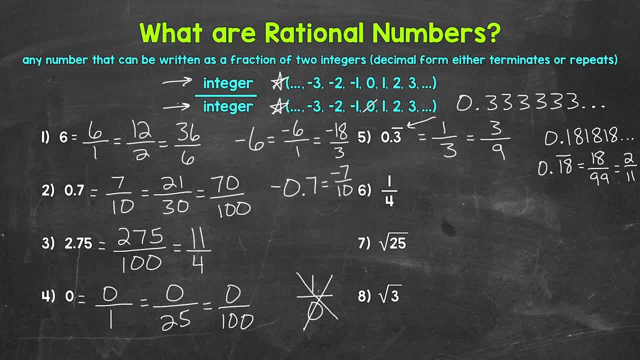 which is an integer, And the denominator is four, which is an integer, So this is rational. Now let's look at the decimal. So we have a terminating decimal form as well. One fourth equals 25 hundredths, which is a terminating decimal. So we can see that this is a rational number that way as well. Let's move on to 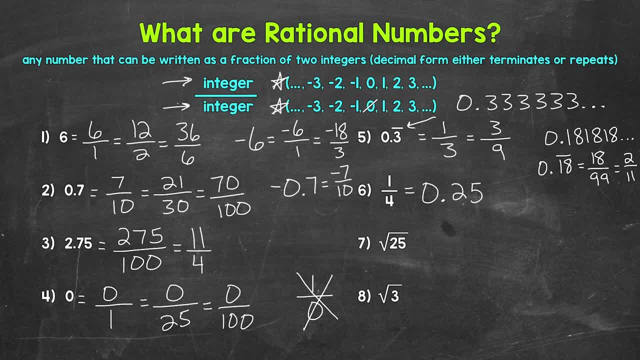 number seven, where we have the square root of 25.. Well, the square root of 25, that equals five. So, with the square root of 25, giving us the value of five, is five rational? Yes, it is. So we have a. 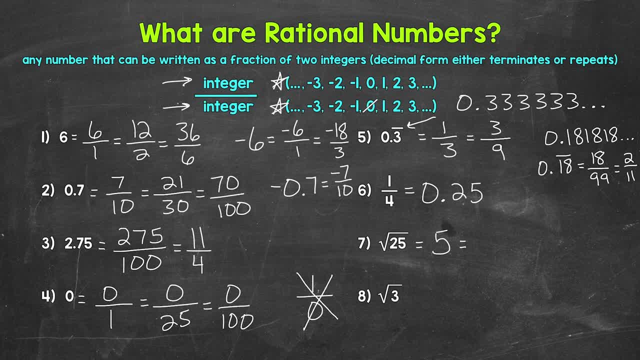 five is a whole number and we can write it as a fraction of two integers: Five over one, 50 over 10, so on and so forth. So the square root of 25 is rational. Lastly, let's move on to. 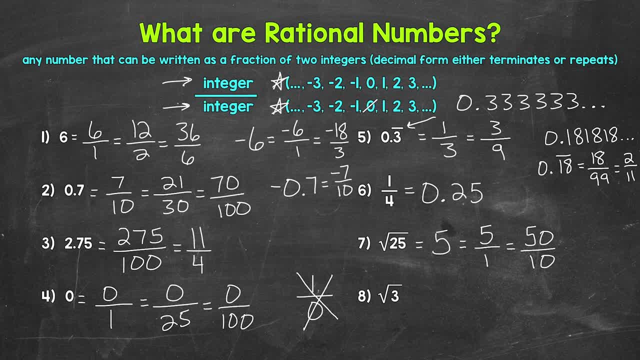 number eight, And at this point you may be thinking: well, what's an example of something that's not rational? Well, the square root of three gives us a value that is not rational. If we plug this into a calculator, we get: 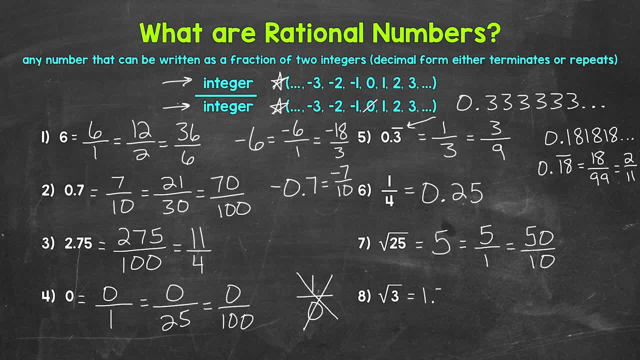 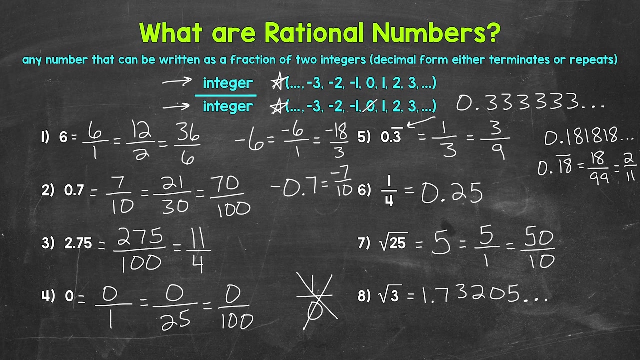 1.73205, and this continues on forever. Now this decimal does not repeat, It doesn't have a pattern, And again, it continues on forever. So the decimal form doesn't terminate or repeat. So there is no way for us to write this as a fraction of two integers. 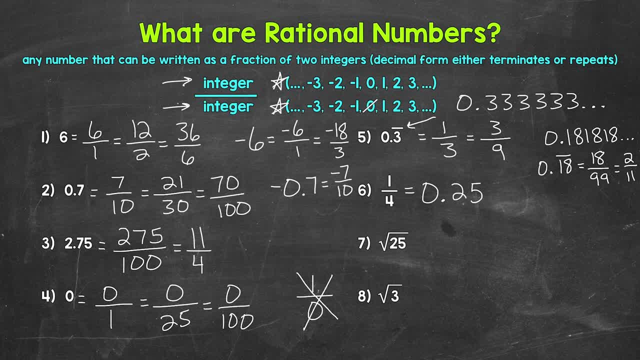 terminating decimal. So we can see that this is a rational number that way as well. Let's move on to number seven, where we have the square root of 25.. Well, the square root of 25, that equals five. So, with the square root of 25 giving us the value of five, 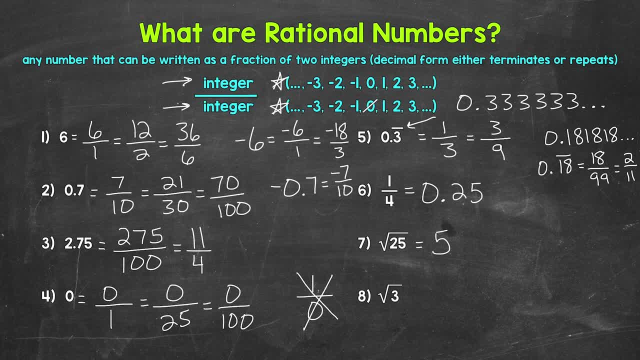 is five rational. Yes, Five is a whole number and we can write it as a fraction of two integers: Five over one, 50 over 10, so on and so forth. So the square root of 25 is rational. Lastly, let's move on to number eight, And at this point you may be thinking well. 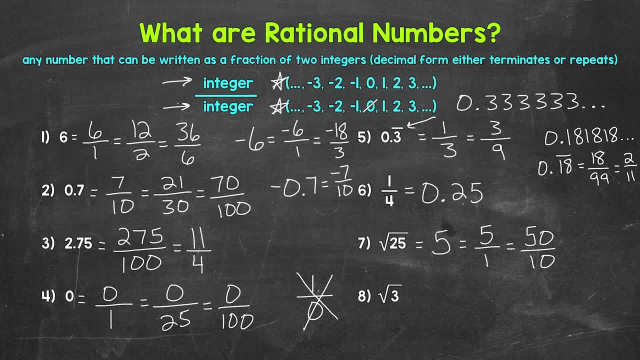 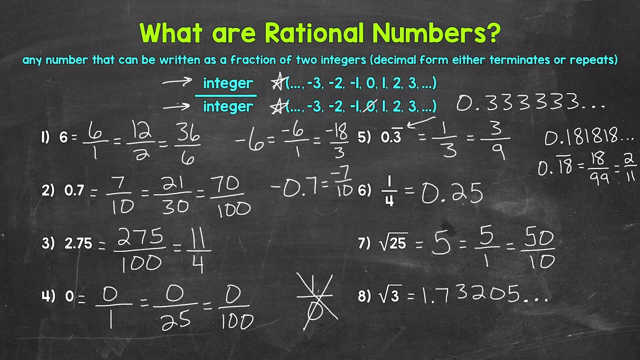 what's an example of something that's not rational? Well, the square root of three gives us a value that is not rational. this into a calculator, we get 1.73205, and this continues on forever. Now this decimal does not repeat, It doesn't have a pattern. and again, it continues on forever. So the decimal form doesn't. 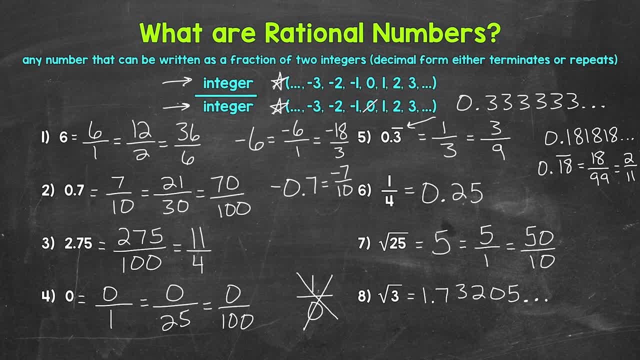 terminate or repeat. So there is no way for us to write this as a fraction of two integers. So this is not rational. Again, there's no way for us to write this as a fraction of two integers. But you may be thinking: can't we just write this as the square root of 3 over 1?? That's a fraction, Yes, it. 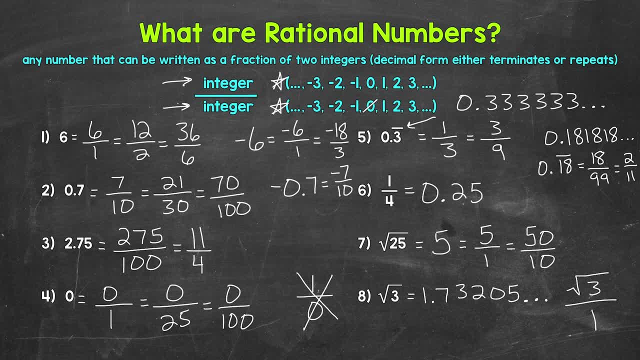 is a fraction. but remember, a rational number is any number that can be written as a fraction of two integers. This numerator is not an integer. Again, the numerator and denominator have to be an integer for it to be rational. The square root of 3 is not rational. It's what we call irrational. We 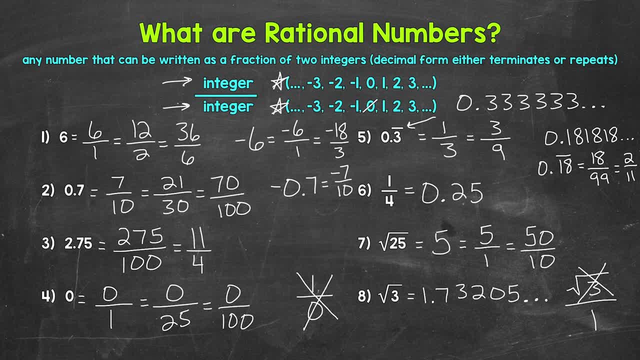 cannot write it as a fraction of two integers, And going off of this anytime, we take the square root of something that is not a perfect square, or a cube root of something that is not a perfect cube, and so on. We can't write it as a fraction of two integers, So we have to write it as a 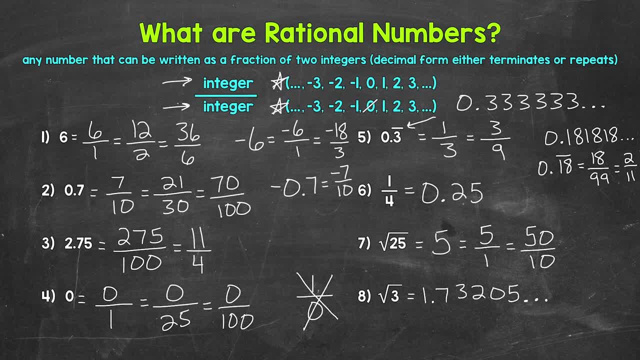 So this is not rational. Again, there's no way for us to write this as a fraction of two integers. But you may be thinking: can't we just write this as the square root of three over one? That's a fraction. Yes, it is a fraction, But remember, a rational number is any number that. 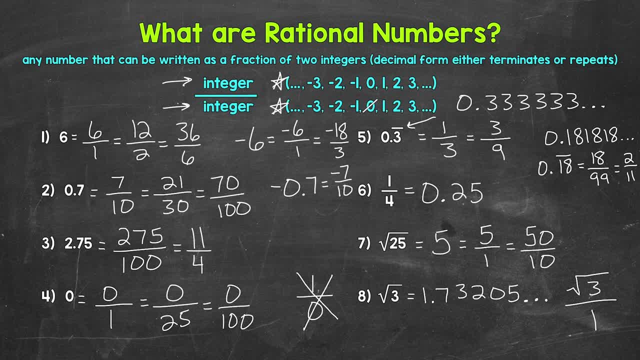 can be written as a fraction of two integers, And this numerator is not an integer. Again, the numerator and denominator have to be an integer for it to be rational. The square root of three is not rational. It's what we call irrational. We cannot write it as a fraction. 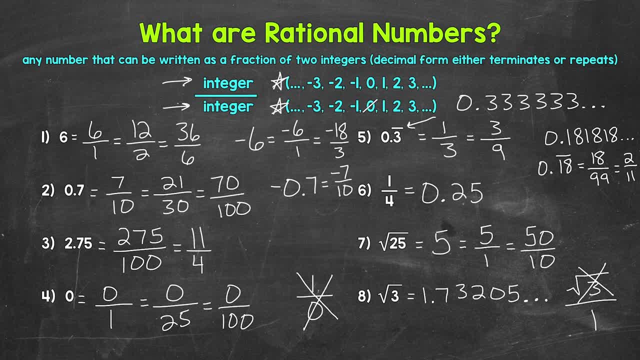 of two integers And going off of this, any time we take the square root of something that is not a perfect square, or a cube root of something that is not a perfect cube, and so on, we get an irrational number. And there are other examples of the square root of three, but I'm not going to. 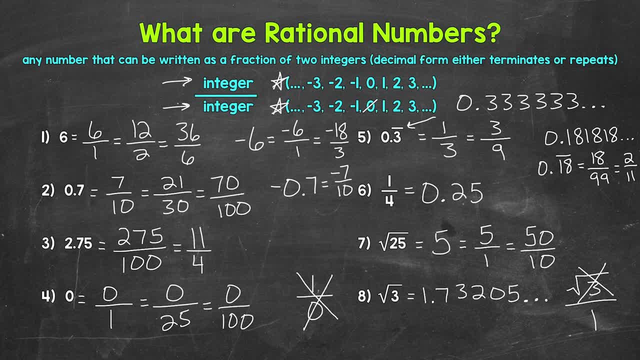 go into the details of irrational numbers as well. We will go over those in another video. That link is down in the description. So as far as rational numbers go, if we can write it as a fraction of two integers, then that number is rational. 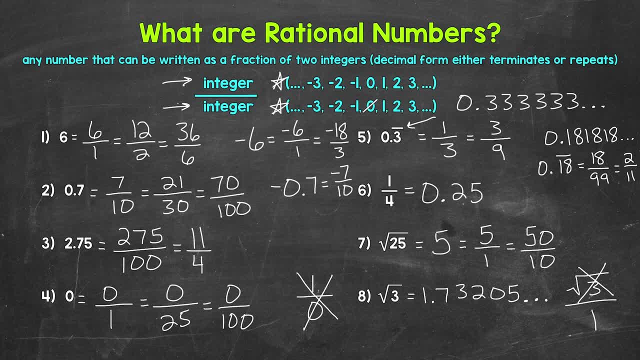 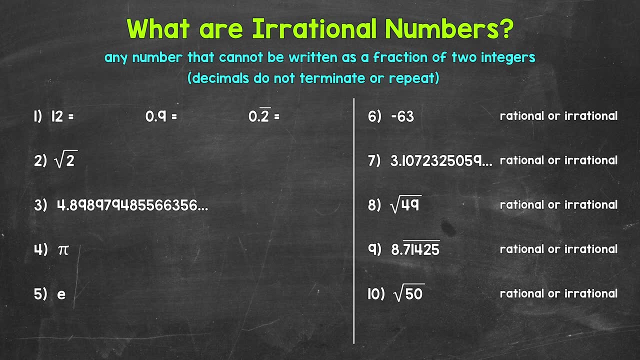 If the decimal form either terminates or repeats, that also shows that we have a rational number. There's a basic overview of rational numbers. Let's move on to irrational numbers. So here is our irrational numbers section. But before we move on to irrational numbers, 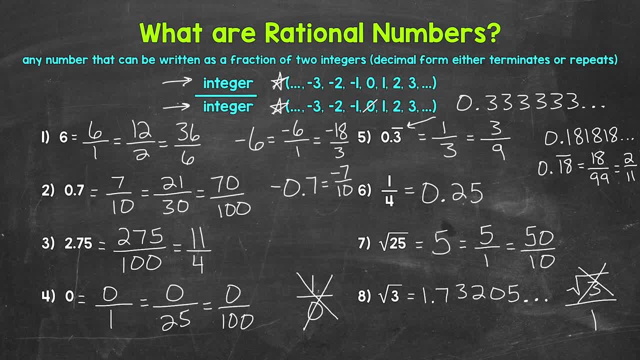 rational number. And there are other examples of irrational numbers as well. We will go over those in another video. That link is down in the description. So as far as rational numbers go, if we can write it as a fraction of two integers, then that number is rational. If the decimal form 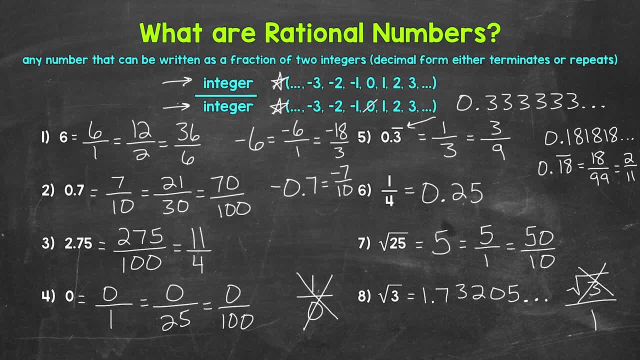 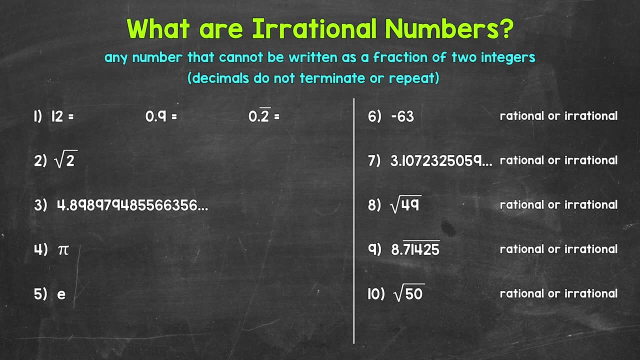 either terminates or repeats. that also shows that we have a rational number. There's a basic overview of rational numbers. Let's move on to irrational numbers. So here is our irrational numbers section. But before we move on to irrational numbers, let's do a quick recap of 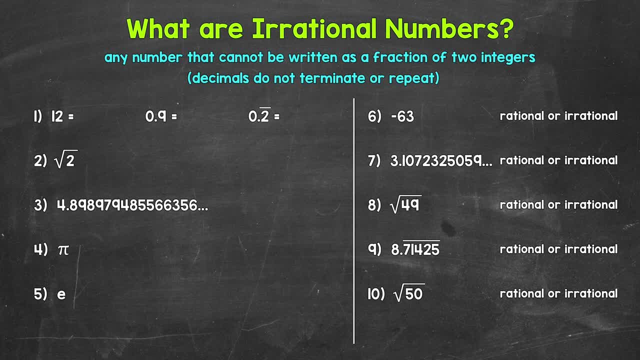 rational numbers, Just to make sure we have those down. So, taking a look at number one, we have 12, 9 tenths and 0.2 repeating. These are all rational numbers. We can write them as fractions, Fractions of two integers. 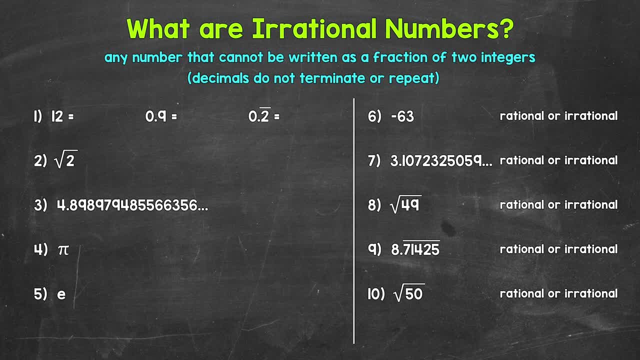 let's do a quick recap of rational numbers, just to make sure we have those down. So, taking a look at number one, we have 12,, 9 tenths and 0.2 repeating. These are all rational numbers We can. 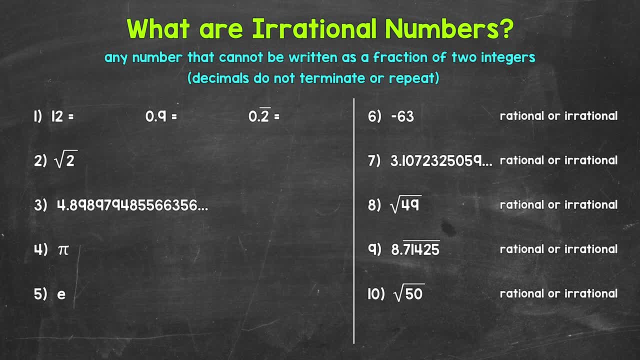 write them as fractions: fractions of two integers And the decimal form of a rational number either terminates or repeats. So if we take a look at number one, we have 12,, 9 tenths and 0.2 repeating. So for 12,, how can we write this as a fraction of two integers? Well, we can write this as: 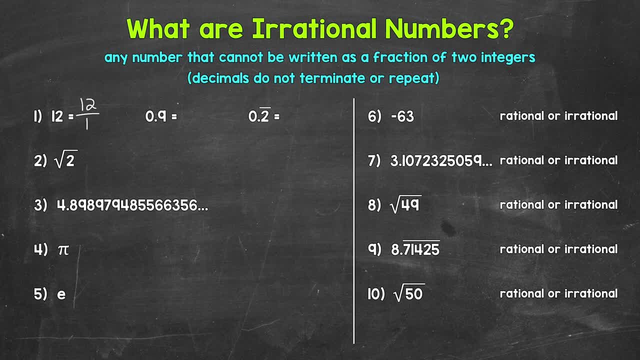 12 over 1. That equals 12.. How about 24 over 2?? That equals 12.. And so on. So we can write 12 as a fraction of two integers. So it is rational. And the same thing goes for. 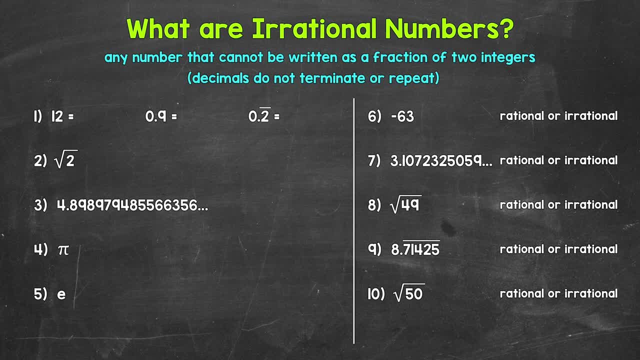 And the decimal form of a rational number either terminates or repeats. So for 12, how can we write this as a fraction of two integers? Well, we can write this as 12 over 1. That equals 12.. About 24 over 2. That equals 12.. And so on. So we can write 12 as a fraction of two integers. So it is. 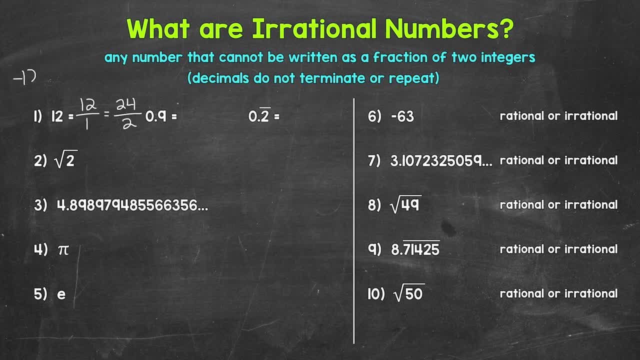 rational. And the same thing goes for negative 12.. So it doesn't matter if we have a negative, This is still rational. We can write this as negative 12 over 1. And so on. So negative 12 is also rational. Let's move on to 9 tenths. 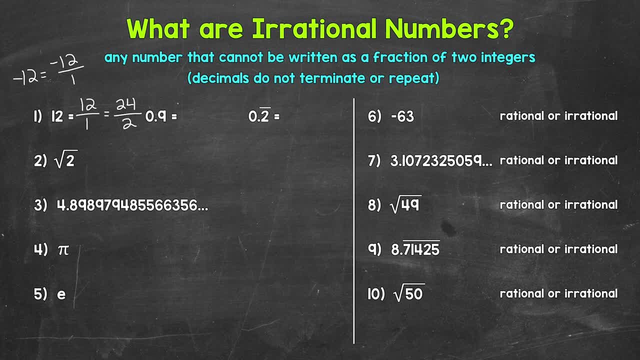 Now this is a terminating decimal, So we can see that this is rational right away. But as far as writing this as a fraction of two integers, we can write this as 9 over 10. Or even something like 6 over 40. And so on. So we can write this as a fraction of two integers. 9 tenths is rational. 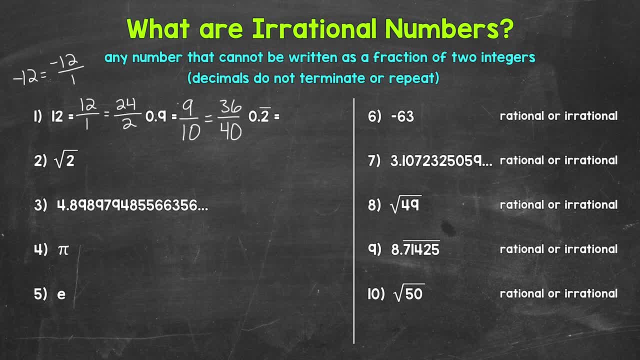 And then, lastly, we have 0.2. repeating This bar over the 2 means we have 0.2222.. And this continues on forever. Now, any repeating decimal is rational. It can be written as a fraction of two integers. 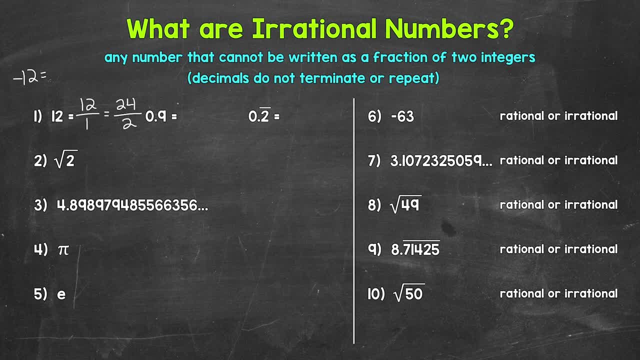 negative 12.. So it doesn't matter if we have a negative. This is still rational. We can write this as negative 12 over 1, and so on. So negative 12 is also rational. Let's move on to nine-tenths. 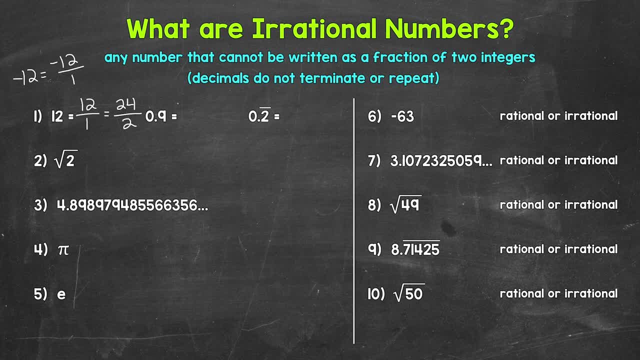 Now, this is a terminating decimal, so we can see that this is rational right away. But as far as writing this as a fraction of two integers, we can write this as 9 over 10, or even something like 36 over 40 and so on. So we can write this as olsun. We can write this as Será. 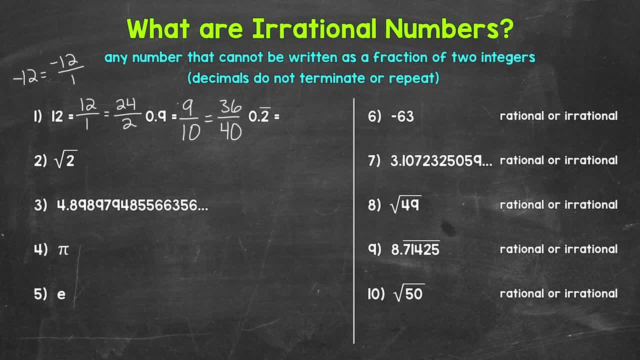 fraction of two integers, 9 tenths, is rational. And then, lastly, we have 0.2. repeating This bar over the 2 means we have 0.2222, and this continues on forever. Now, any repeating decimal is rational. It can be written as a fraction. 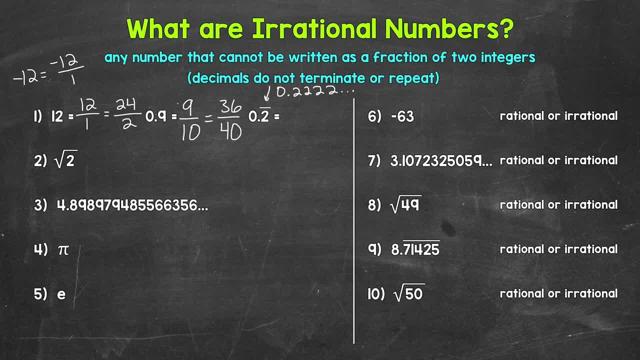 of two integers, For example 0.2, repeating can be written as 2 over 9 or 6 over 27, and so on. Let's move on to irrational numbers and we will start with the square root of 2.. Now, the square root of 2 is approximately so. 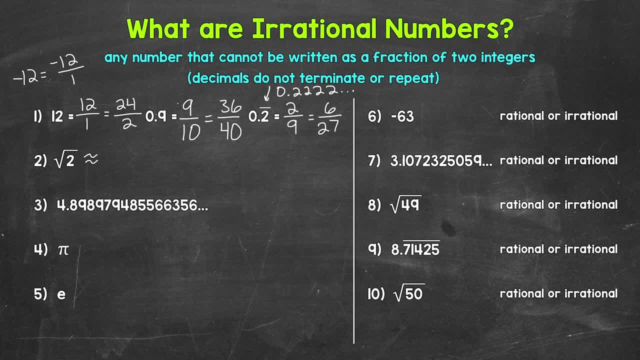 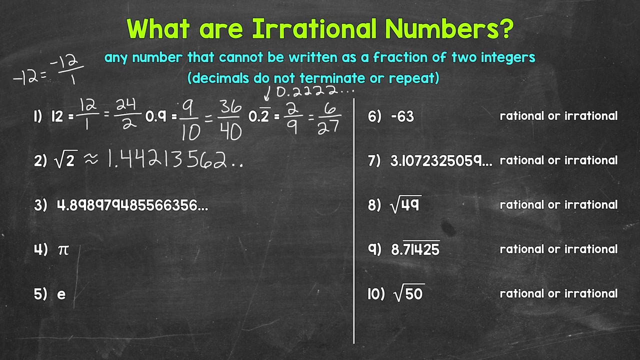 let's put approximately- and I say approximately because this decimal does not terminate or repeat, so we can't write out the full decimal- So the square root of 2 is approximately 1.4422, 1, 3,, 5,, 6,, 2, and this continues on. Again, it does not terminate or repeat, So this 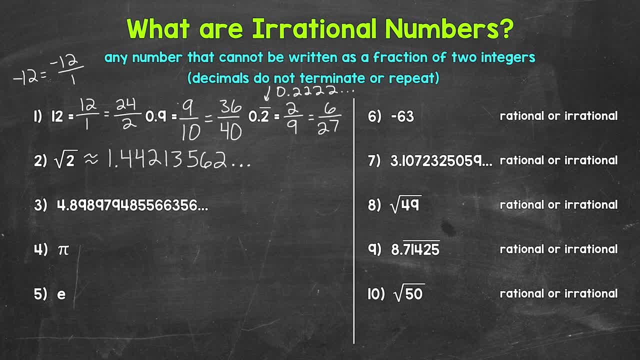 is irrational. There's no way to write this as a fraction of two integers. Now you may be thinking: well, let's just write it as the square root of 2 over 1.. Yes, it is a fraction, but it has to be a fraction of two integers. 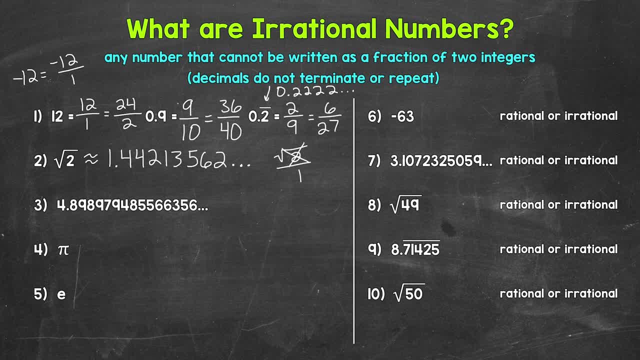 The square root of 2 is not an integer. So again, we cannot write the square root of 2 as a fraction of two integers and the decimal doesn't terminate or repeat. This is actually going to be the case for taking the square root of anything. 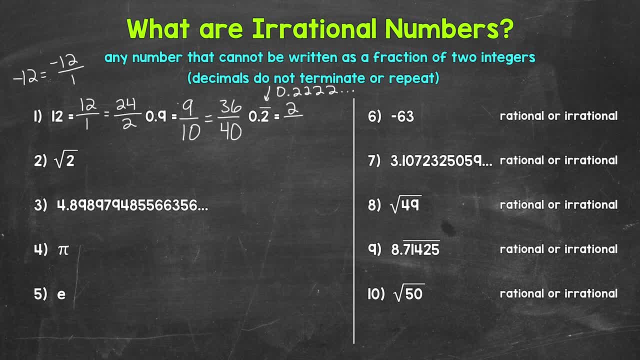 For example, 0.2 repeating Can be written as 2 over 9. Or 6 over 27. And so on. Let's move on to irrational numbers And we will start with the square root of 2.. Now the square root of 2 is approximately, So let's put. 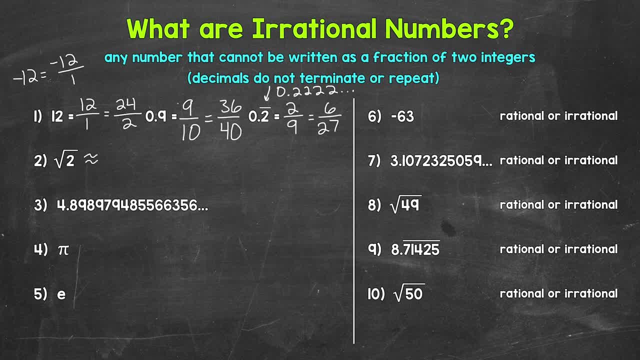 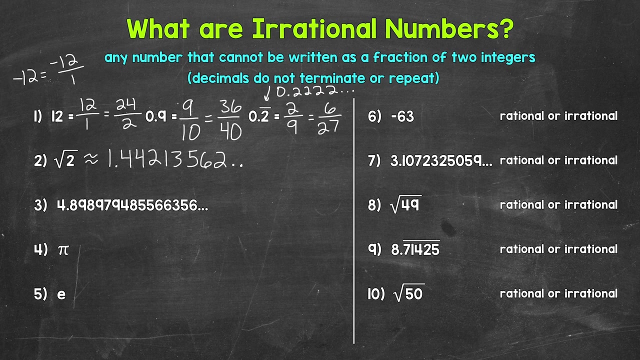 approximately. And I say approximately because this decimal does not terminate or repeat, So we can't write out the full decimal. So the square root of 2 is approximately 1.4.. 4., 2., 1., 3., 5., 6., 2.. And this continues on. Again, it does not terminate or repeat, So this is. 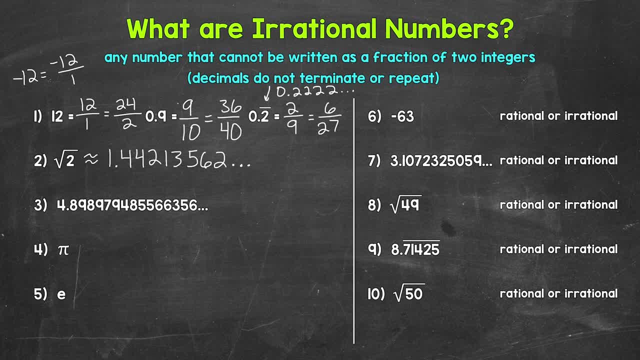 irrational. There's no way to write this as a fraction of two integers. Now you may be thinking: well, let's just write it as the square root of 2 over 1.. Yes, it is a fraction of two integers, But it has to be a fraction of two integers. The square root of 2 is not an integer. So again we 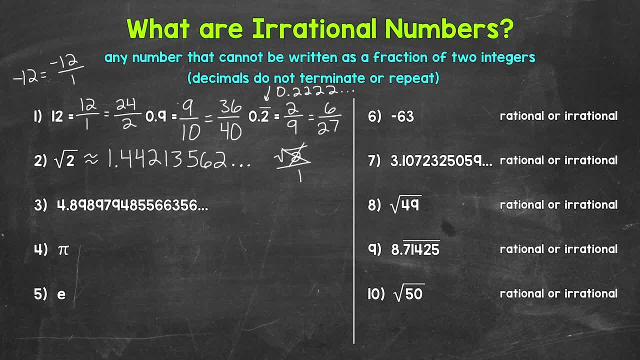 cannot write the square root of 2 as a fraction of two integers And the decimal doesn't terminate or repeat. This is actually going to be the case for taking the square root of anything that is not a perfect square, So the square root of any non-perfect square is irrational. Let's move on to 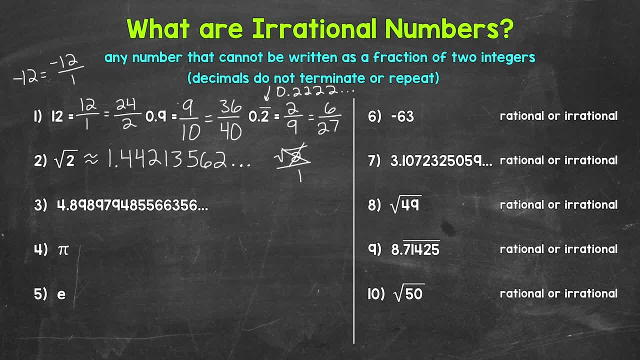 4.89897948.. And then that decimal continues on. It does not terminate or repeat. So this is irrational. We cannot write this as a fraction of two integers. Now, this decimal is actually what we get when we plug in the square root of 24 into a calculator. Next, for number four, we have pi. 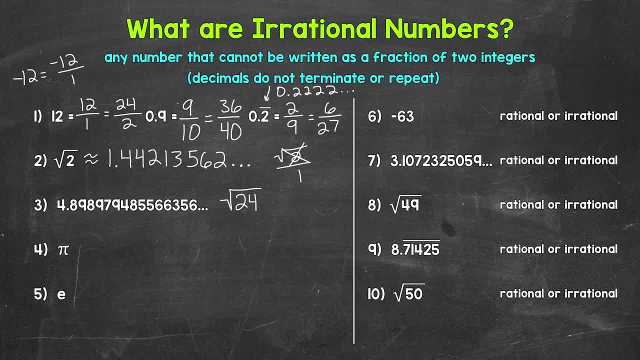 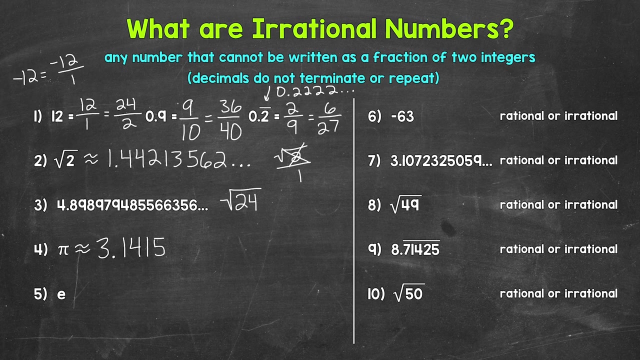 Which is a very famous irrational number that we use when working with circles. Pi is the ratio of a circle's circumference to its diameter. So the circumference divided by the diameter, Pi is the same for every circle. Now pi is approximately 3.1415926.. And this 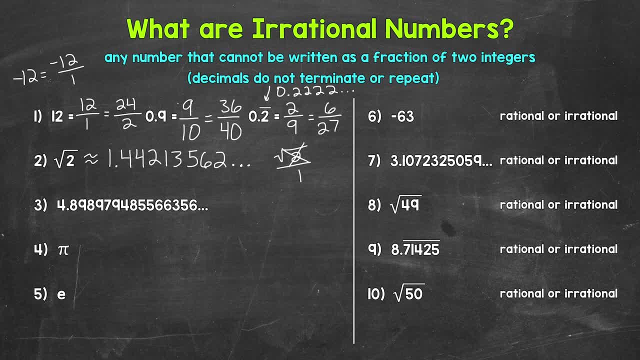 that is not a perfect square, So the square root of any non-perfect square is irrational. Let's move on to number 3, where we have 4.898979.. 4, 8, and then that decimal continues on. It does not terminate or repeat. So this is. 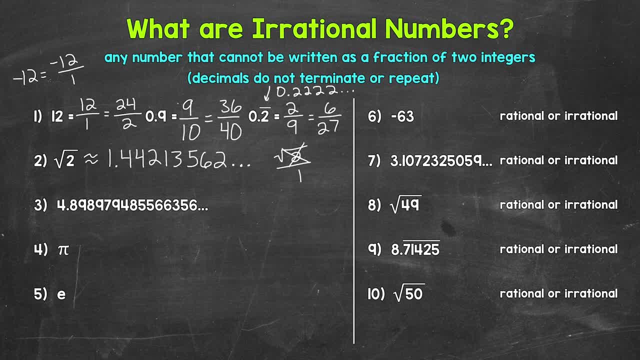 irrational. We cannot write this as a fraction of two integers. Now, this decimal is actually what we get when we plug in the square root of 24 into a calculator. Next, for number four, we have pi, which is a very famous irrational number that we use. 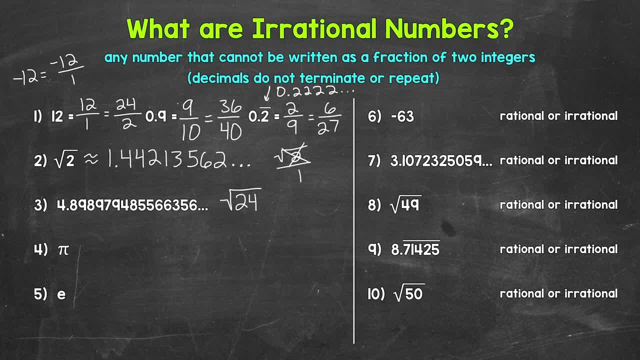 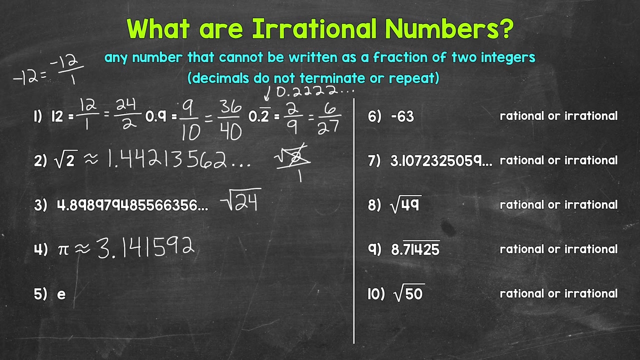 when working with circles. Pi is the ratio of a circle's circumference to its diameter. So the circumference divided by the diameter, Pi is the same for every circle. Now pi is approximately 3.1415926, and this continues on forever, without repeating. 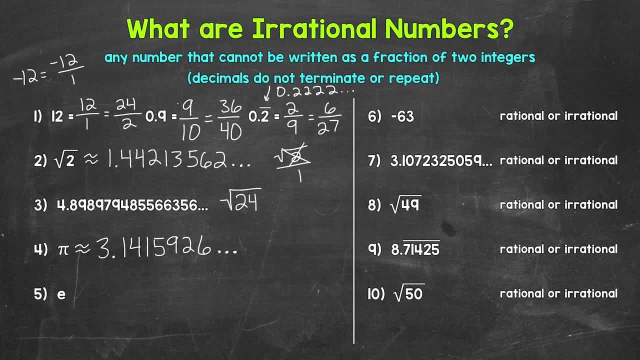 Now we cannot write pi as a fraction of two integers. Pi is irrational. Now it's very common to use 3.14 for pi, but that's just an approximation. Let's move on to number five, where we have the number e, also called Euler's number, named after the mathematician Leonard Euler. This is another. 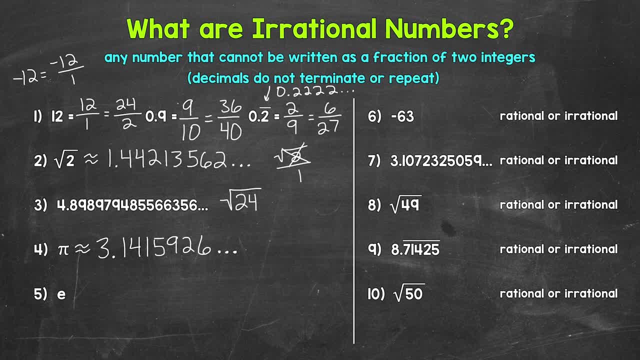 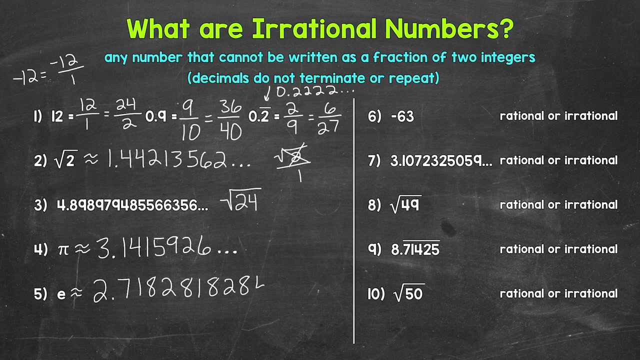 famous irrational number that shows up throughout math with things like exponential growth, compound interest probability, among other applications. The number e is approximately 2.71828182845, and this continues on forever without repeating, So we can't write the number e. 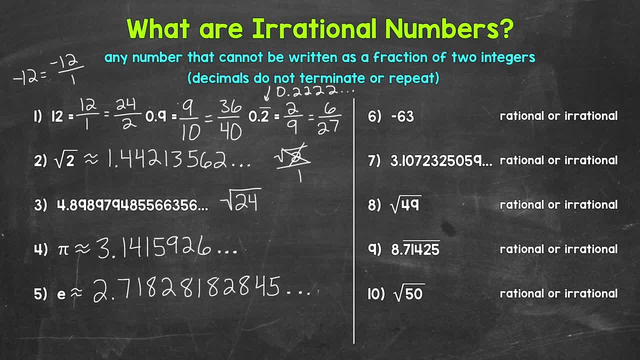 as a fraction of two integers. It's irrational. Now let's move on to numbers six and seven. Pi is approximately 3.1415926, and this continues on forever without repeating. Now we cannot write pi as a fraction of two integers. Pi is on its original value, which is: 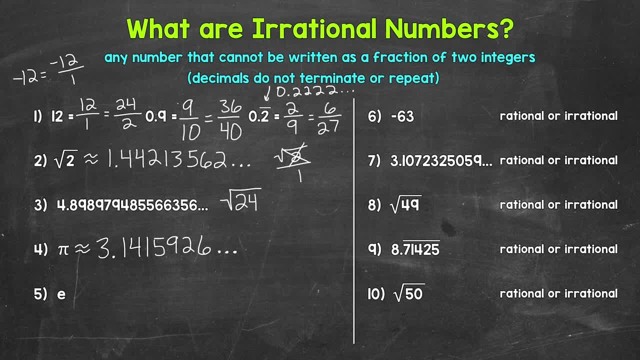 continues on forever without repeating. Now we cannot write this as a fraction of two integers. Pi is irrational. Now it's very common to use 3.14 for pi, But that's just an approximation. Let's move on to number five, where we have the number e, Also called Euler's number, Named after 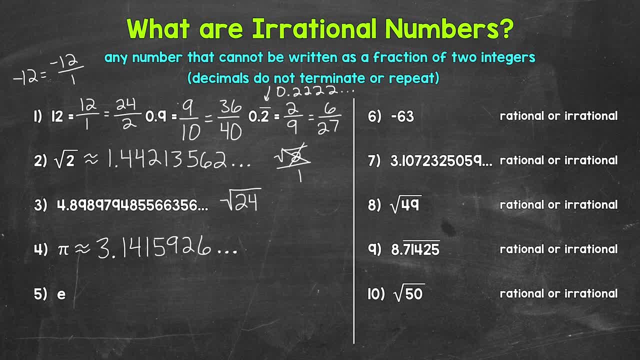 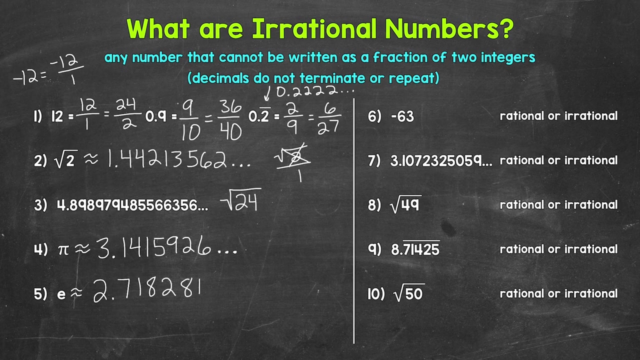 the mathematician Leonard Euler. This is another famous irrational number that shows up throughout math, With things like exponential growth, compound interest probability, among others. The number e is approximately 2.71828182845.. And this continues on forever, without repeating. 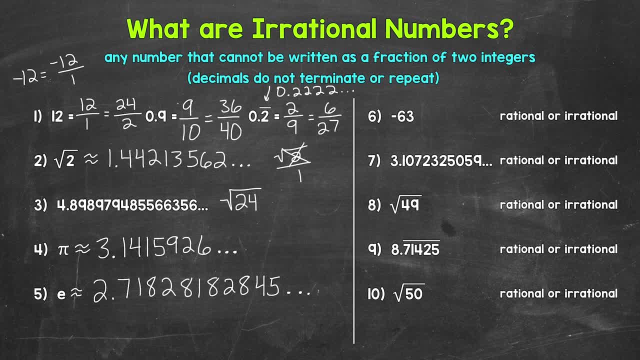 So we can't write the number e as a fraction of two integers. It's irrational. Now let's move on to number seven, where we will determine if we have something that is rational or irrational. For number six, we have negative 63.. This is rational. We can write this as a fraction of two integers. 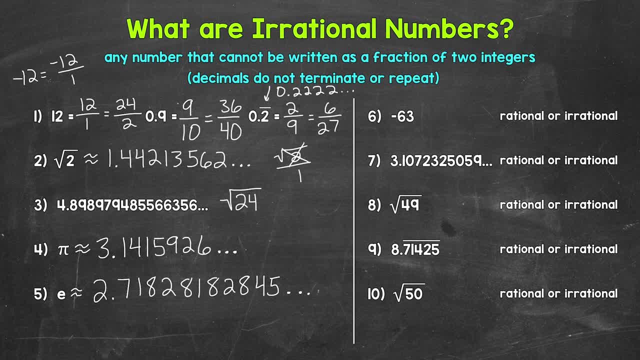 For example, negative 63 over 1.. So negative 63 over 1.. Again, this is rational. Next, for number seven, we have 3.107234.. And this is a fraction of two integers, So we can write this as a fraction of two. 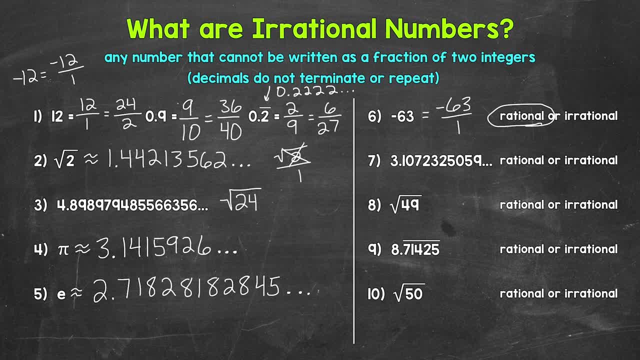 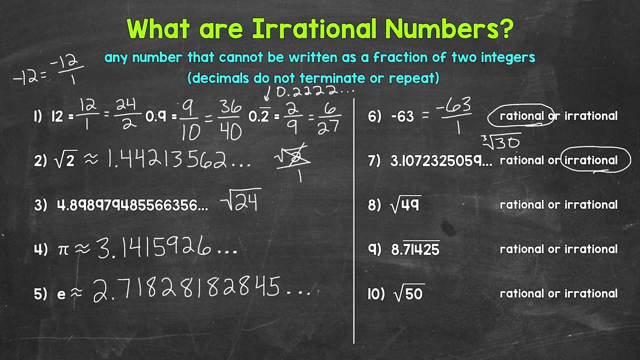 integers. This is irrational. We can't write it as a fraction of two integers. This is actually the decimal that we get for the cube root of 30.. So this is irrational. Next, let's move on to number eight, where we have the square root of 49.. Now, 49 is a perfect square, So the square root of 49. 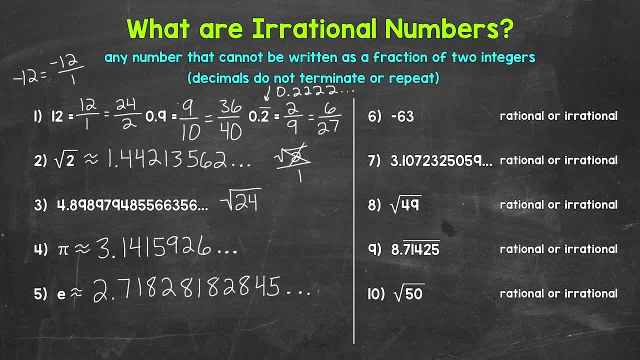 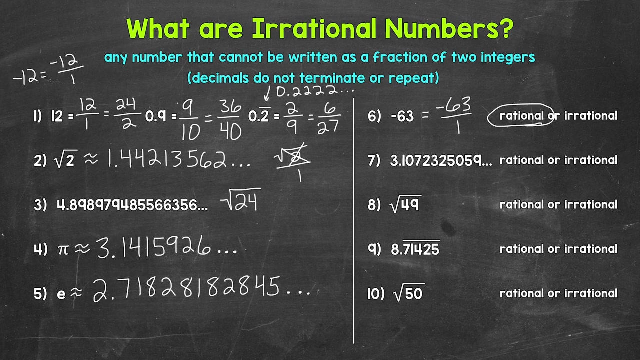 pi. It's the same County here. Then let's write some calculations down to the entire area of. we have thorista when we write our bättre 3.10723, and that decimal continues on without terminating or repeating. This is irrational. 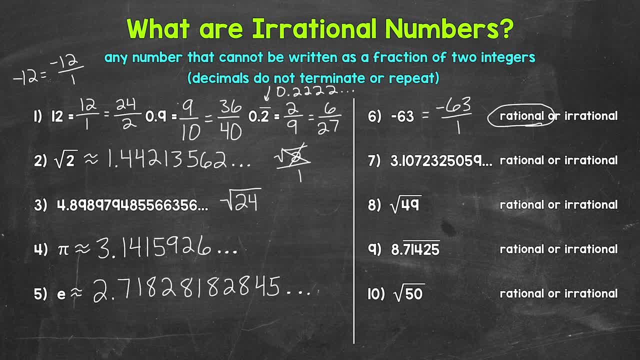 We can't write it as a fraction of two integers. This is actually the decimal that we get for the cube root of 30.. So this is irrational. Next, let's move on to number eight, where we have the square root of 49.. Now, 49 is a perfect square, So the square root of 49. 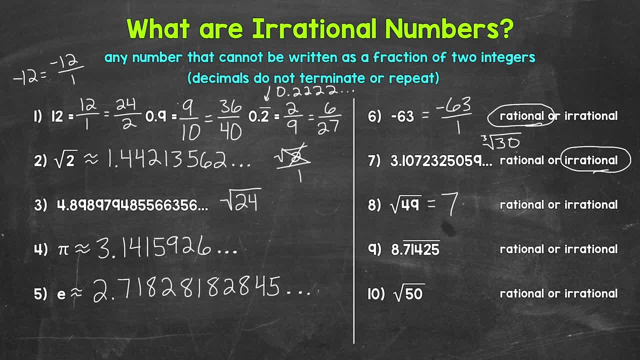 equals 7.. So the square root of 49, rational. Moving on to number nine, we have 8.71425.. Now, above 71425, we have a bar That shows us that that decimal repeats, And again, any repeating decimal. 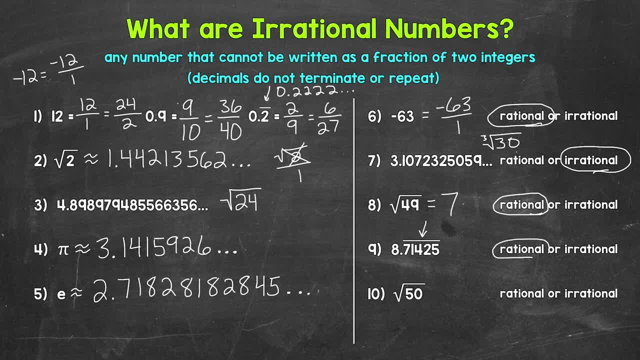 is rational, So this is rational. Lastly, let's move on to number 10, where we have the square root of 50.. 50 is not a perfect square, So this is not going to work out to be a rational number. The square root of 50 is approximately 7.07106.. And this continues on forever. 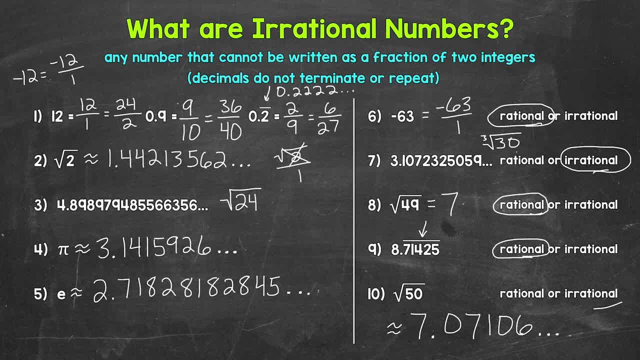 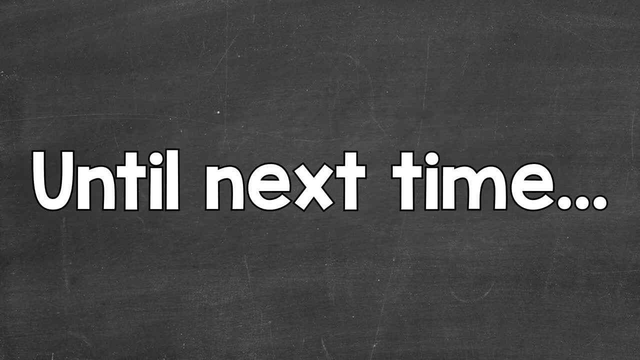 without terminating or repeating. So the square root of 50 is irrational. So there you have it. There's an introduction to rational numbers and irrational numbers. I hope that helped. Thanks so much for watching. Until next time, peace. 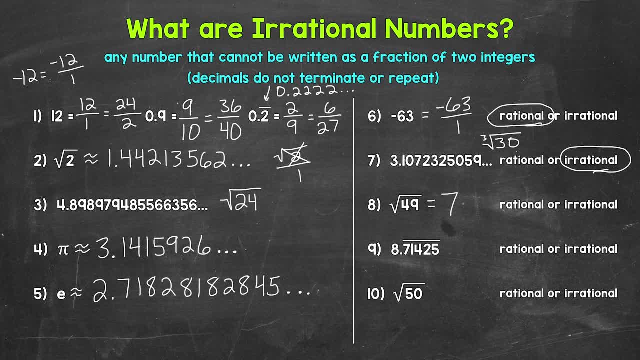 equals 7.. So the square root of 49 is rational. Moving on to number nine, we have 8.71425.. Now, above 71425, we have a bar That shows us that that decimal repeats. And again, any repeating decimal is rational. So this is rational. Lastly, let's move on to number ten, where we can write this: 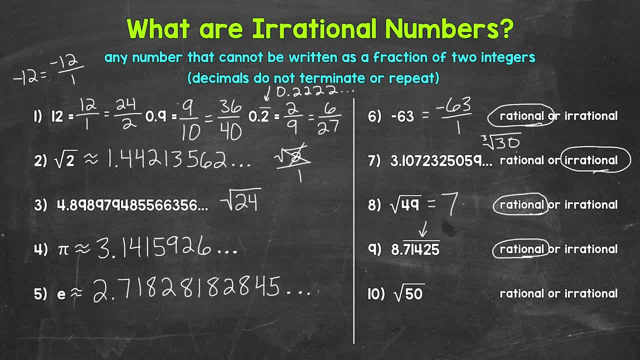 as a fraction of two integers. Here we have 10, 9, 9, 3, 4, 6, 7, 8, 5, 4, 6, 7, 6, 4, 8, 4, 1.. So that's the consequence. We can now do the other dash, And I'm going to do 1 like this, 1 like this. 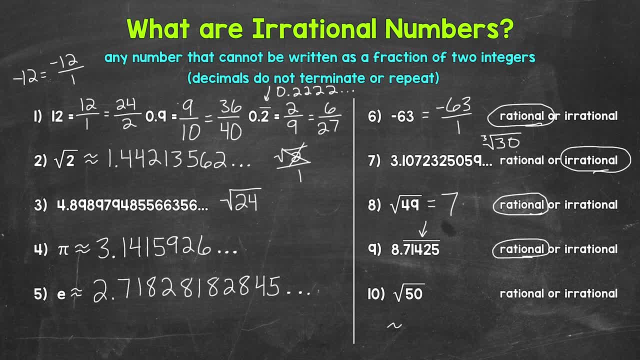 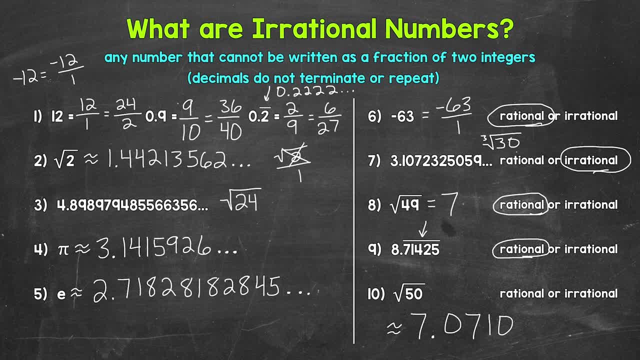 well, Well, I don't have it. yeah, that's not the question there. We know that 2 is a fraction, but we don't know if it's the actual value of 52.. ist's rational, so we don't know. One final: 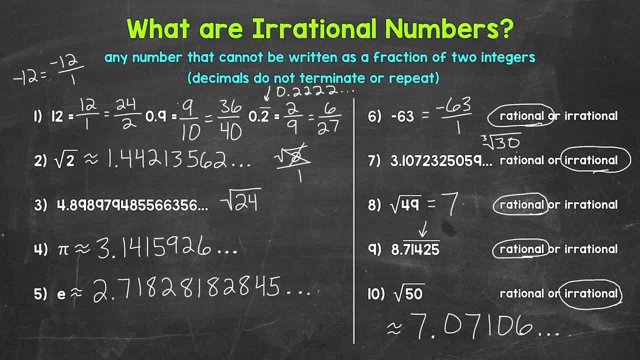 question here. Alright, let's go back to number 3.. Okay, we have Question 24.. And here we have in 대한 stupidovan, It's the'VAAM'. So 2 isn't a fraction of 2.. So I point to number 1 and 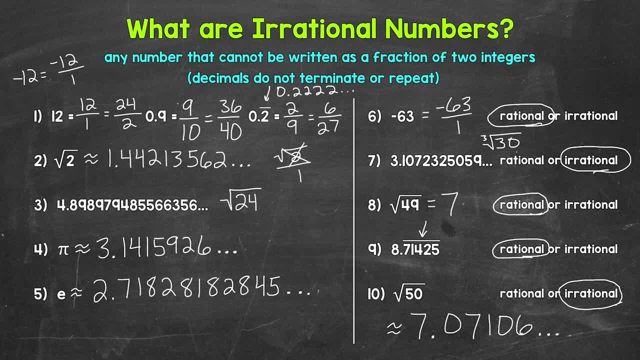 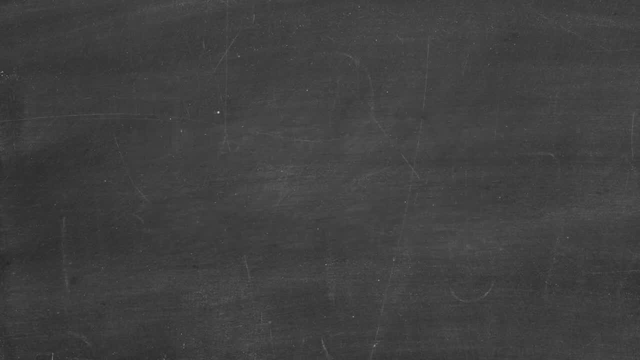 Rational. so there you have it. There's an introduction to rational numbers and Irrational numbers. I hope that helped. Thanks so much for watching. until next time, peace. 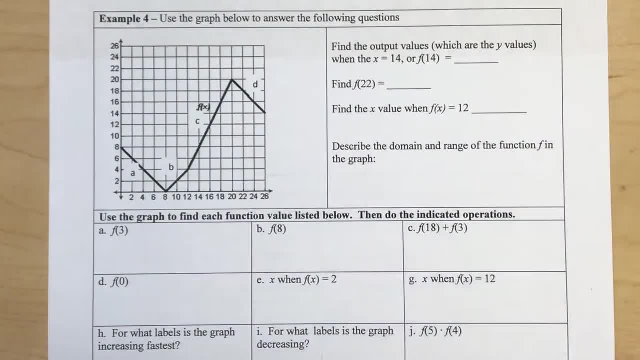 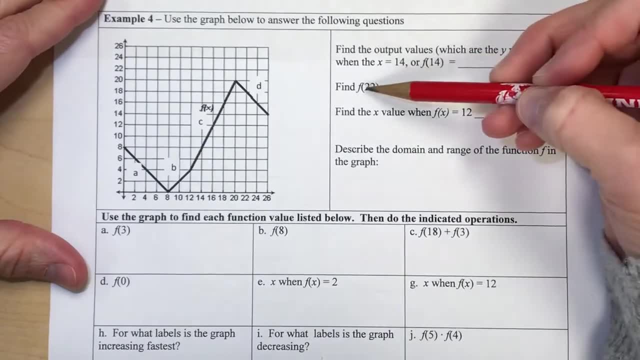 In this video, I am going to show you how to use the graph below to answer the following questions, and what we're going to be doing is evaluating our function based on a couple values that we're given and find either the input that's missing or the output that's missing, according to.